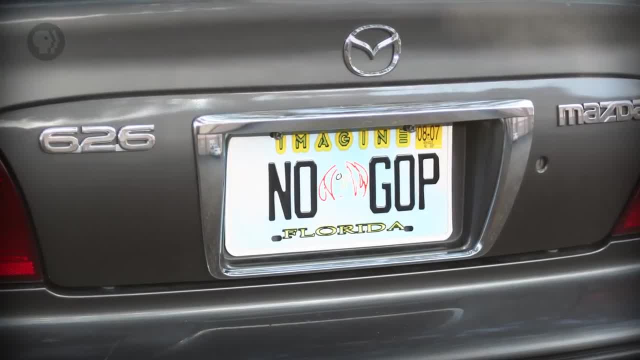 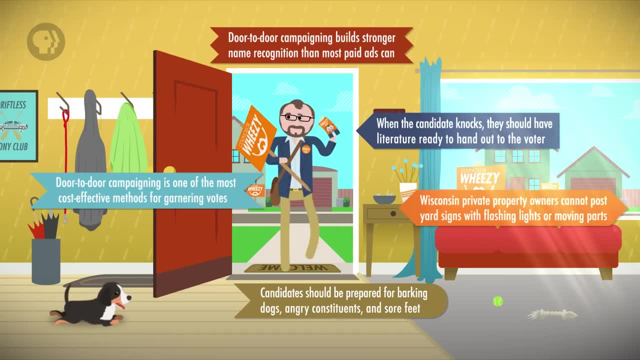 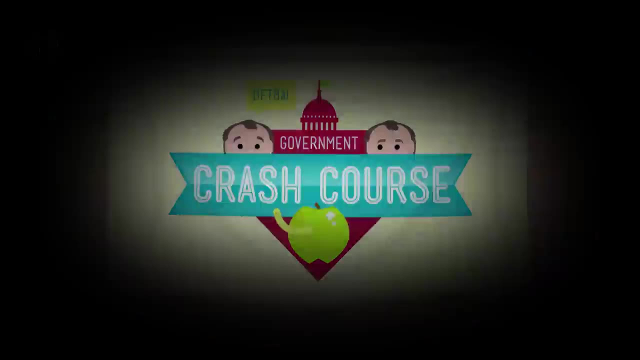 crying. Political ideologies are specific to individuals, but right now we're going to try to explain the factors that shape public opinion in the aggregate, which is a fancy word- for, like all the people, A person's opinions on politics are very much grounded in their ideology, whether they consider 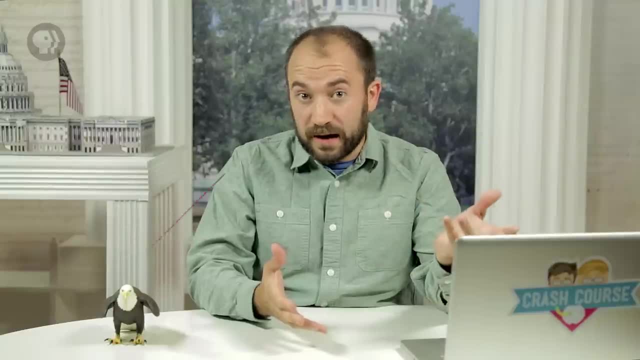 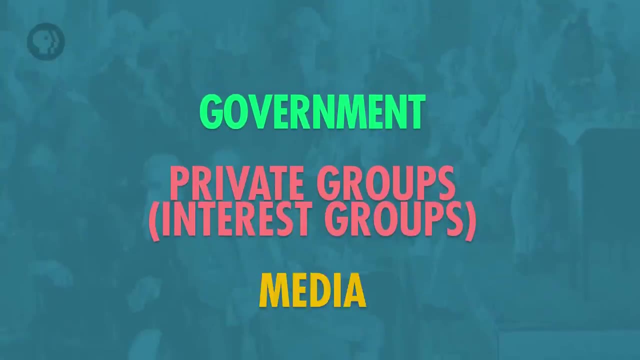 themselves liberal or conservative, but that doesn't mean they aren't susceptible to outside factors. I get my opinions from PewDiePie. Three of the main influences on our political opinions are the government, private groups- aka interest groups- and the media, aka my. 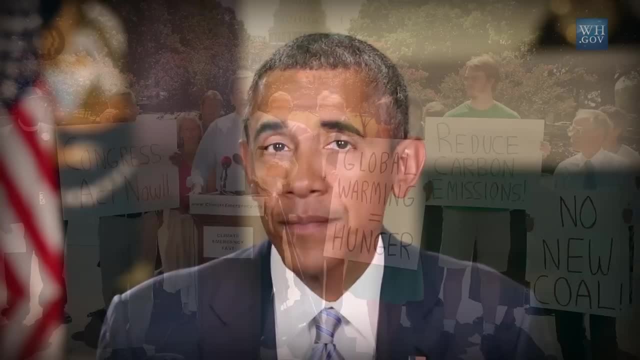 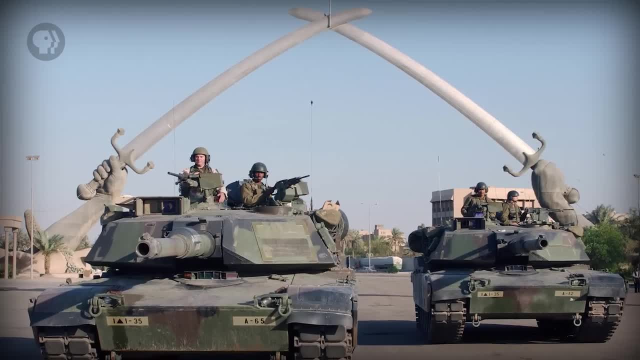 opinion. it's important to know which of these is more effective and, like any political opinion, it's important to know which of these is more effective and like any political taxes or invading other countries. when the government does stuff, we got opinions about it. 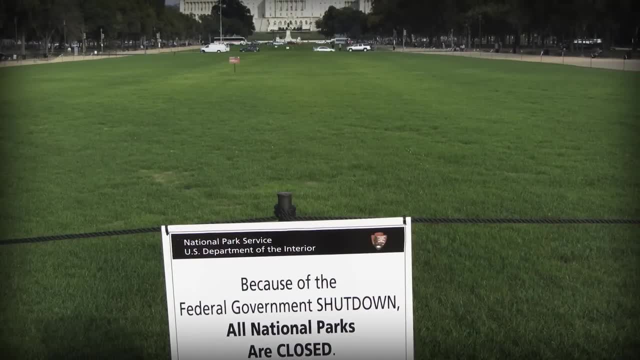 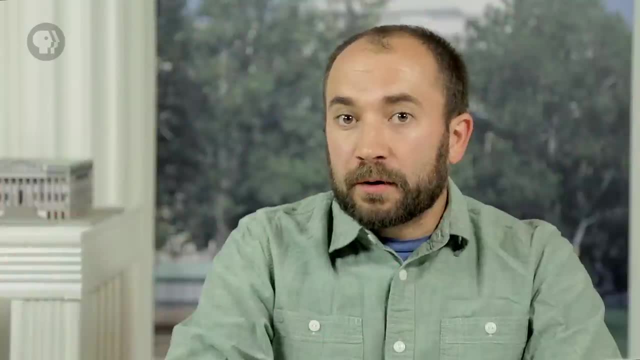 More recently, government inactivity, at least in terms of congressional law-making, has also had an impact on public opinion. It seems like Congress' approval ratings have gotten lower and lower as they pass fewer and fewer bills. But aside from doing or not doing, 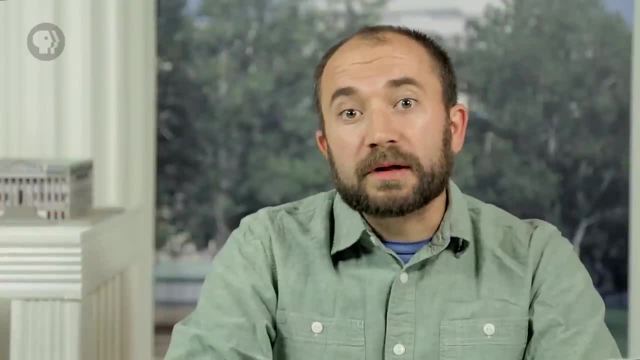 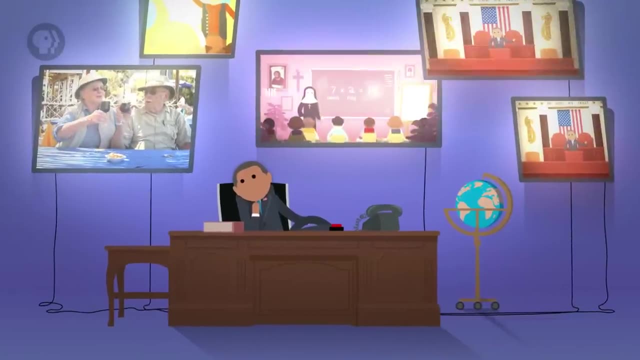 their jobs. the government actively shapes public opinion by engaging in public relations maneuvers and manipulating the news cycle. Let's go to the Thought Bubble. The President is especially good at controlling the news cycle, since he can go on television whenever he wants. The idea that the President might be at the center of the news started. 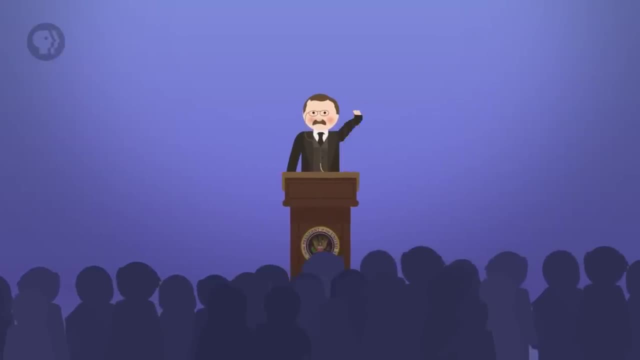 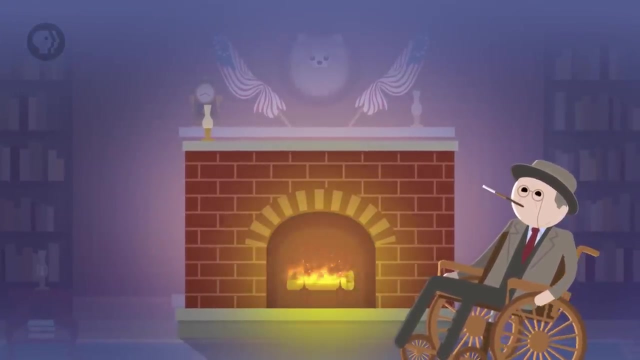 in the 20th century, probably with Theodore Roosevelt, who saw the office of the presidency as a bully pulpit. But it really picked up steam with Franklin Roosevelt, who began the trend of the President speaking directly to the American people with his fireside chats. 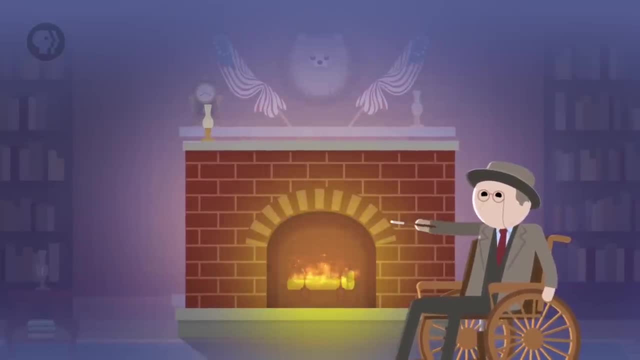 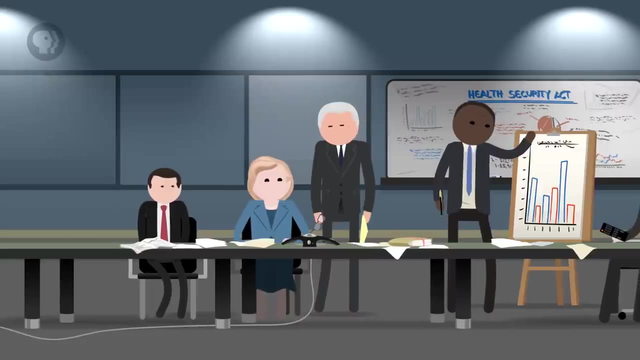 These were direct appeals to Americans to support the President's policies and a classic example of presidential PR. Since then, the government has gotten more sophisticated with its public relations, although perhaps not more effective. President Clinton was known for having a war room to coordinate his PR apparatus. but all the spin in the world didn't. 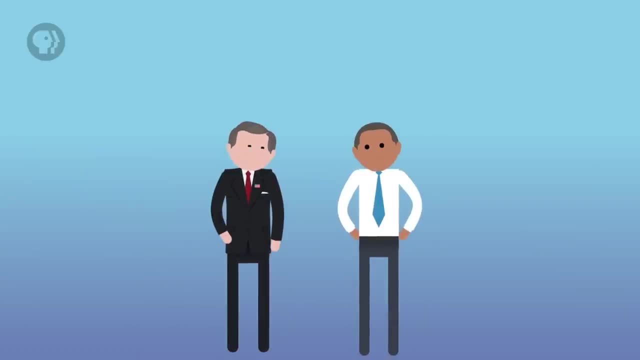 make Americans support his healthcare initiative. Presidents Bush and Obama have continued this team. This is a very popular trend: using public opinion polls to polish their images, even trying to figure out what sort of vacations they should take. But, as with Clinton, there 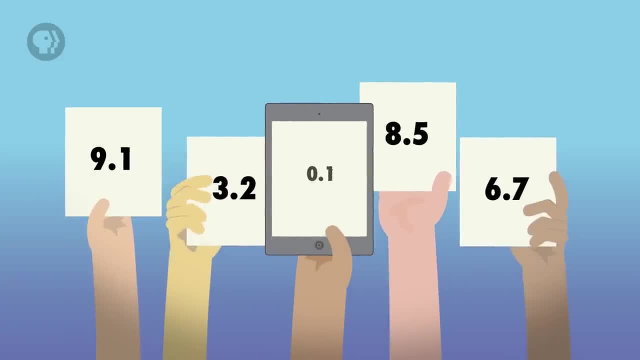 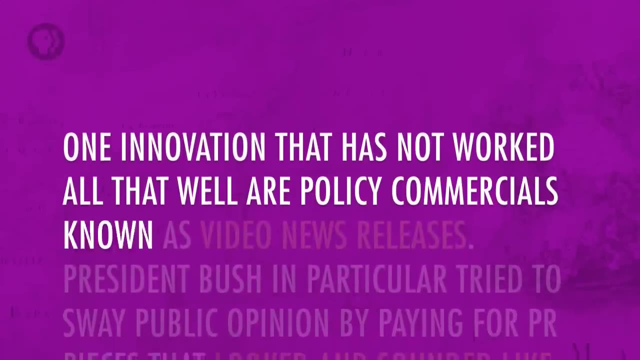 is not a ton of evidence that their PR activities worked. This probably has something to do with the changing media landscape, which we'll discuss in greater detail in future episodes. One innovation that has not worked all that well are policy commercials, known as video news releases. President Bush, in particular, tried to sway public opinion by paying for 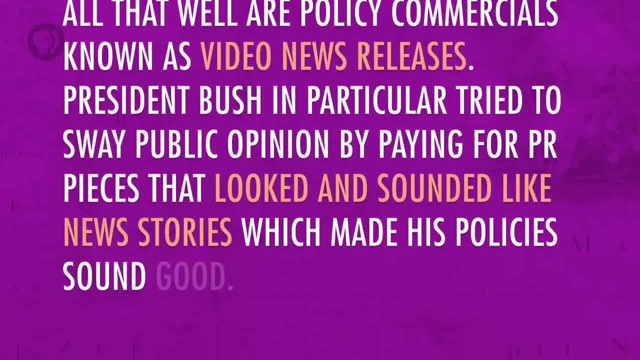 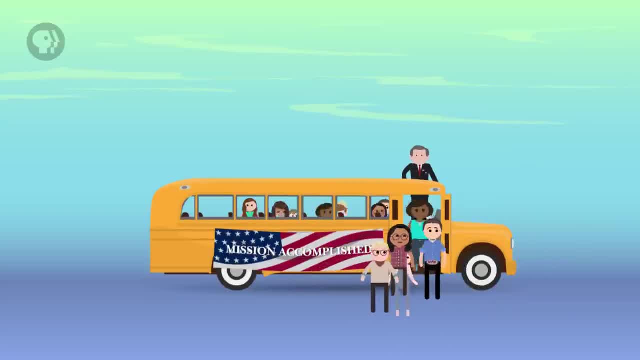 PR pieces that looked and sounded like news stories, which made his policies sound good. This was especially true of his education policies. I'll leave it to you to decide whether you think No Child Left Behind was a success, because the point is that you need to be very careful when watching news stories about 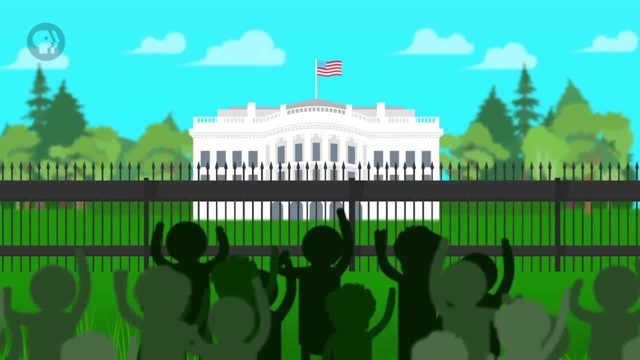 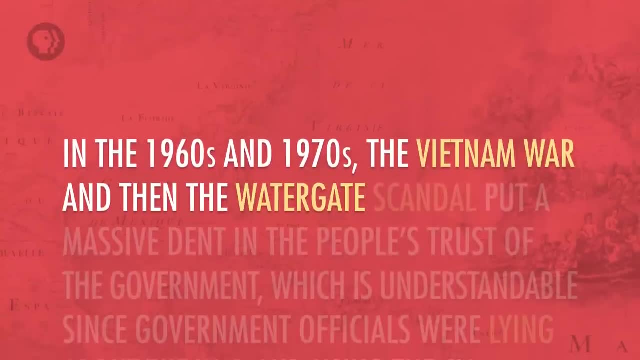 actual policies these days. There's also an historical explanation for why government efforts to create positive public opinion are less successful than we might think. In the 1960s and 1970s, the Vietnam War and then the Watergate scandal put a massive dent in the people's trust of the government. 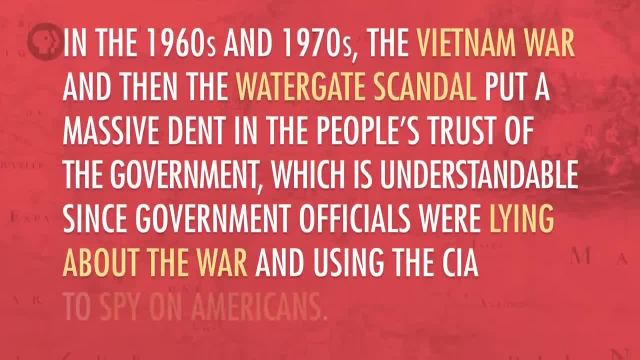 which is understandable, since government officials were lying about the war and using the CIA to spy on Americans. I bet if you ask your parents, or maybe your grandparents, you'll hear a story about how much better the government was back in the 50s and early 60s. But that 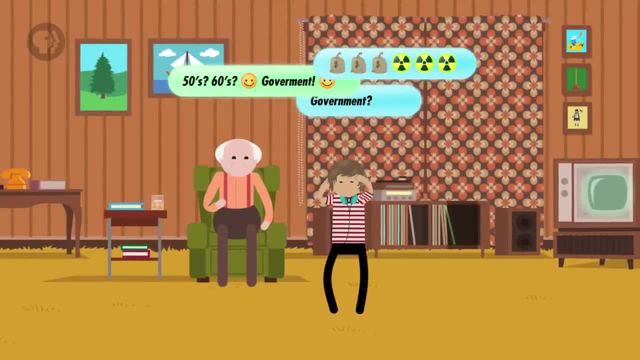 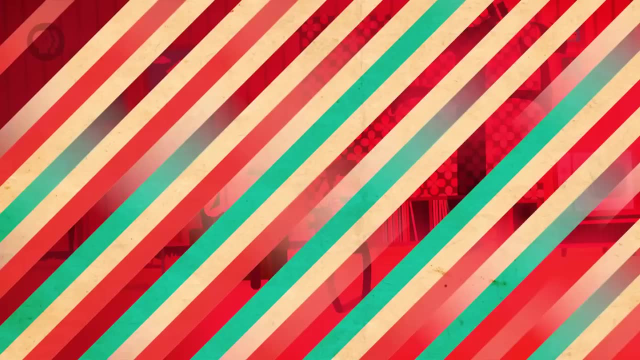 might be a reflection of the generally robust economy and a Cold War consensus That criticizing the government was unpatriotic. you communist sympathizer, And if you're African American, the 1950s and early 1960s probably don't look so rosy either. 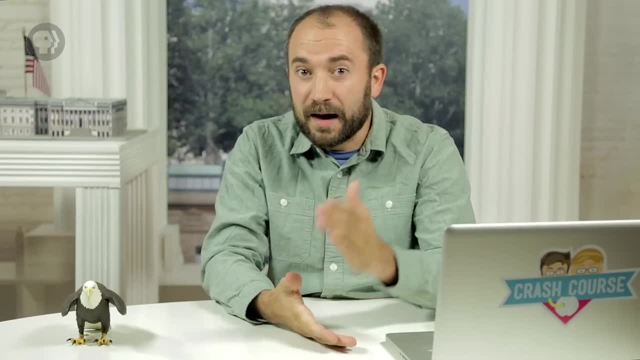 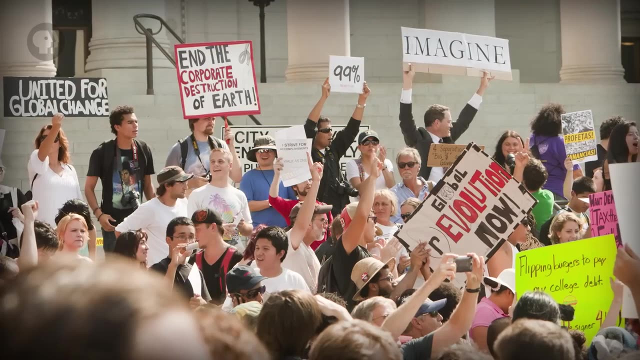 Thanks, Thought Bubble. This brings us to another point about public opinion generally. It's highly reactive to current events, especially the economy, Or eagles being in your vicinity and you wanting to punch them. I don't think it's a coincidence that presidential and congressional approval ratings have been. 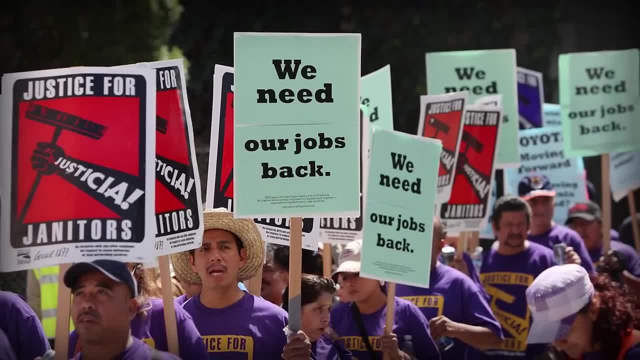 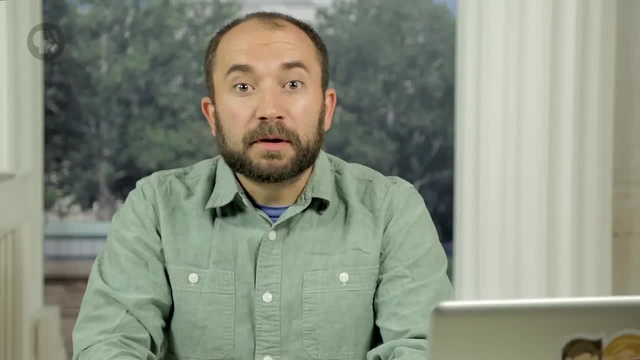 pretty low during the aftermath of the 2008 financial crisis. I mean, Americans love to complain, but the six years following 2008 have seemed pretty awful. Or maybe it has a lot to do with the other two Private groups, especially organized interest groups, but also less formally political organizations. 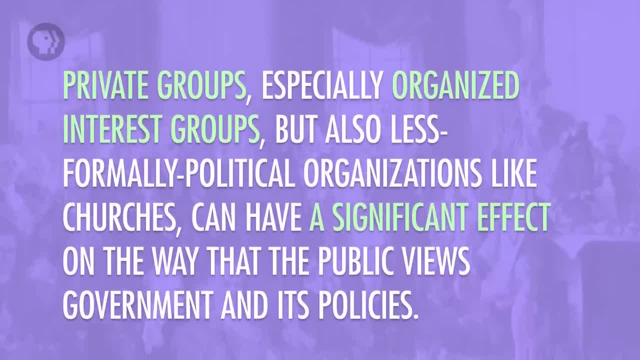 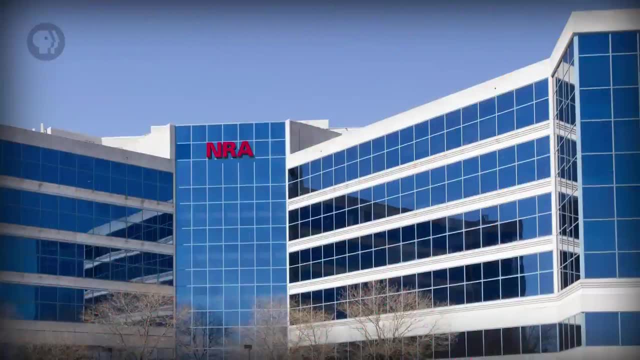 like churches, can have a significant effect on the way that the public views government and its policies. Any group with a particular interest in legislation can mount an advertising campaign for or against a law, provided they have the money to do so. Sometimes, these groups 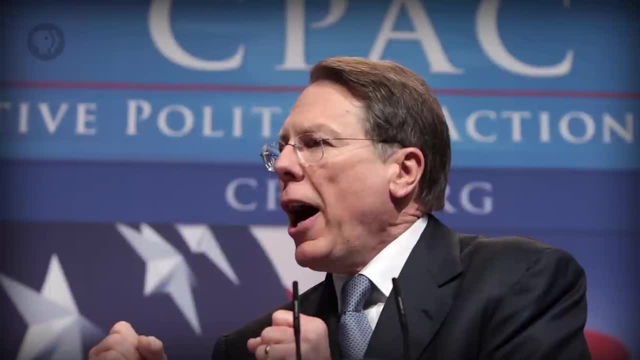 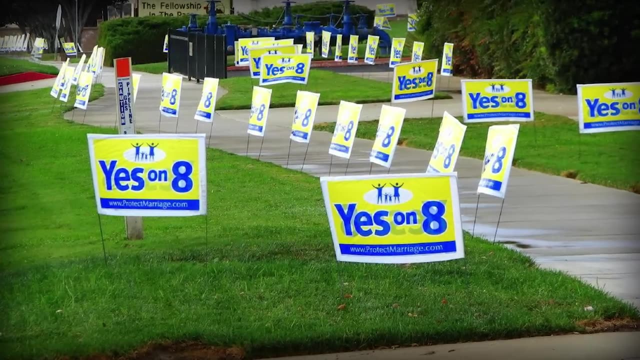 exist already, like the National Rifle Association, which works hard to ensure that stringent regulations on firearms don't get passed. Other times, an interest group will grow up around a specific issue, as often happens in states like California that feature ballot initiatives. The growth of the internet as a source of news, information and advertising has lowered 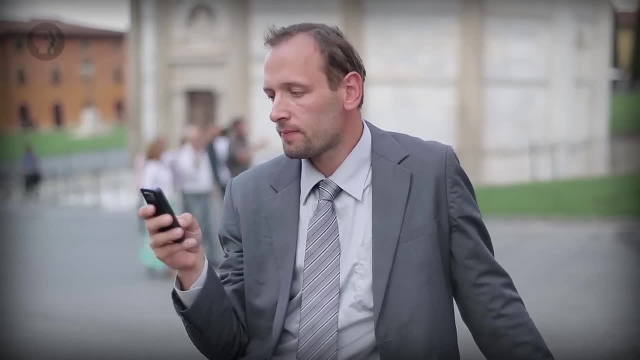 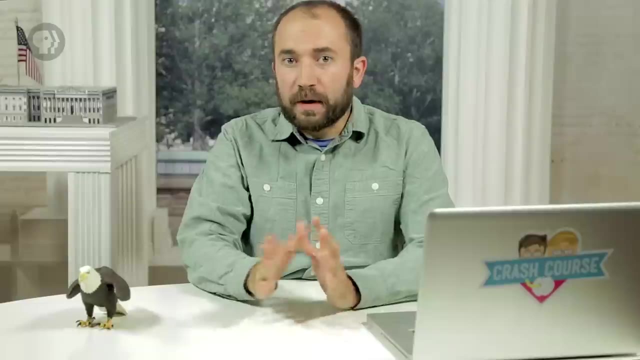 the cost of public relations and makes it easier for specific interest groups to get their messages out, like the time I tumbled about how the dress was totally black and blue. Often the group that's better at swaying public opinion has more money. A great example of how an interest group with a lot of money and a single issue can shape. 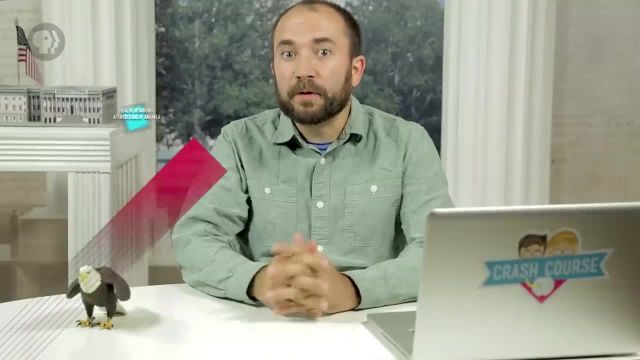 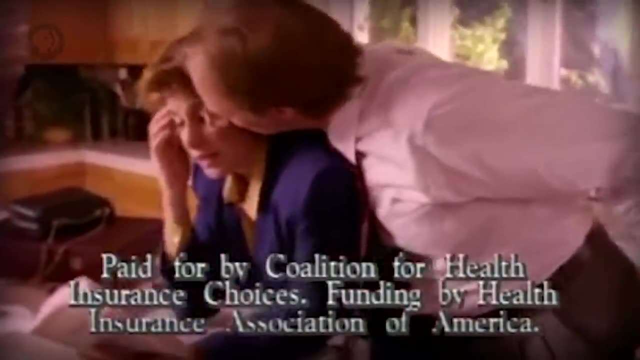 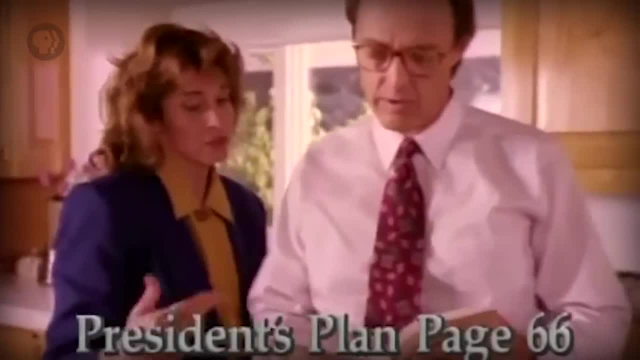 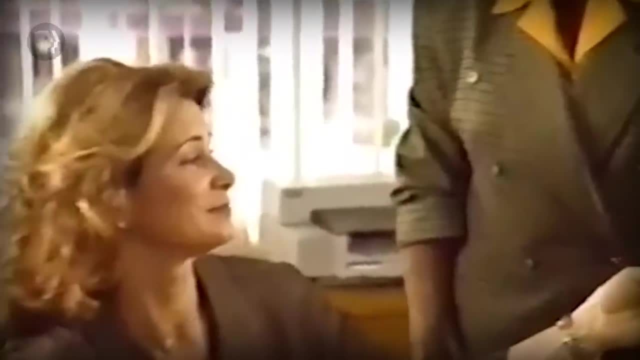 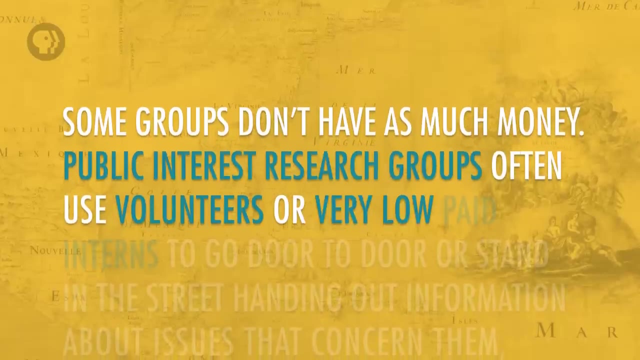 Iש consecretária. The ads cost between 14 and 20 million dollars and are widely credited with helping move public opinion against the Clinton health policy. Some groups don't have as much money- public interest research groups often use volunteers or very low-paid interns to go door to door or stand in the street handing out information. 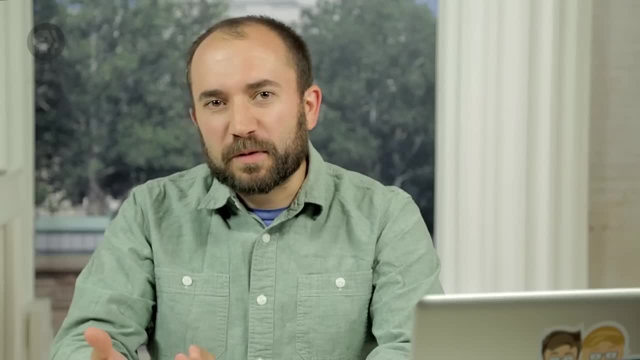 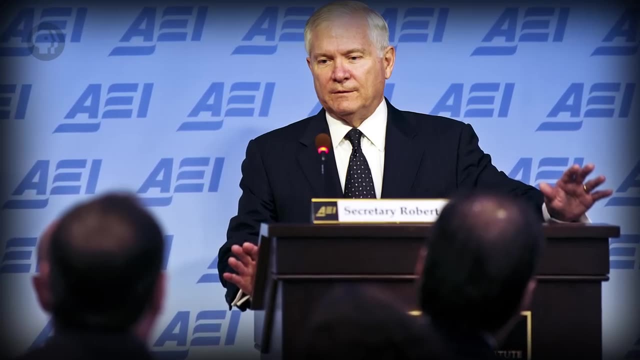 about issues that concern them, such as the environment. Both liberal and conservative groups sponsor think-tanks that produce research intended to change people's minds. On the right are groups like the Heritage Foundation and the American Enterprise Institute. On the left, you might have heard of the Brookings Institute. All the information. 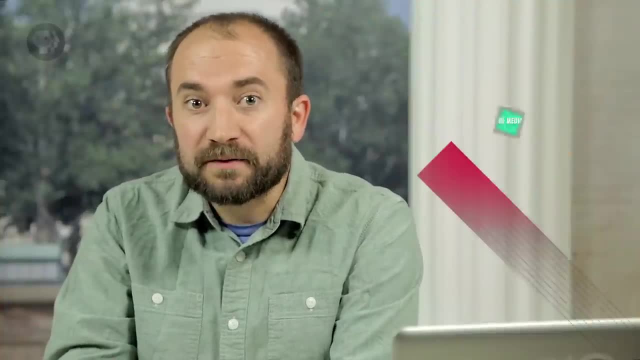 that's put out by various think tanks and interest groups probably wouldn't have as big an impact if not for the third factor: shaping public opinion: the media. Of the three, the media tends to be the most powerful force in shaping public opinion because it's 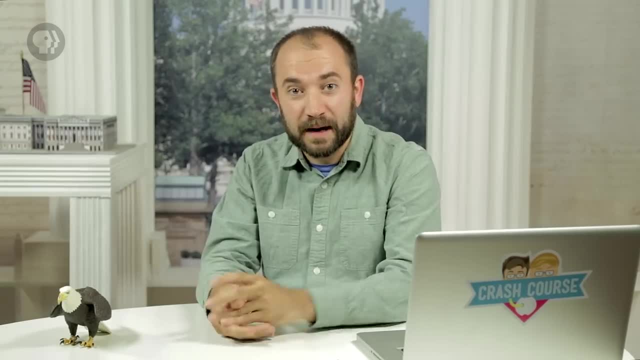 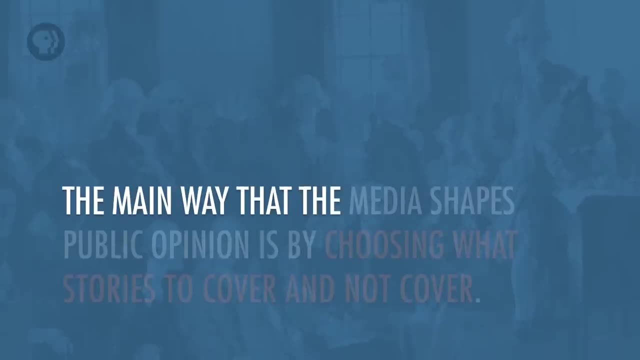 everywhere and it's easy to access, and people look all nice with their makeup and the flashy graphics make them seem real smart. For most of us, the news media is the lowest cost way to get our information that shapes our opinion, The main way that the media shapes public. 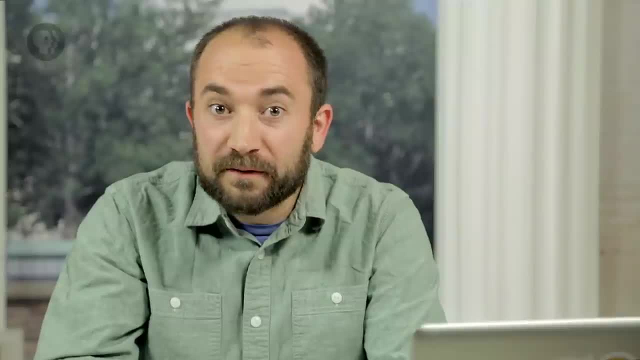 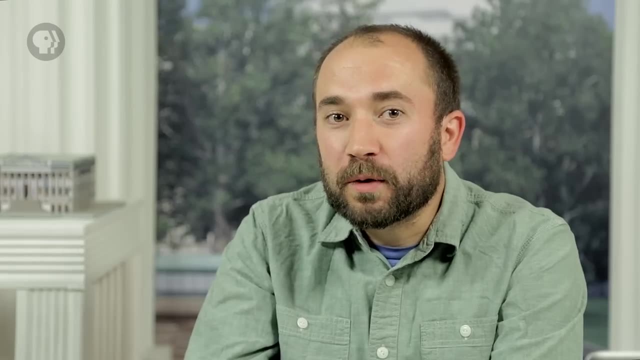 opinion is by choosing what stories to cover and not cover. It's pretty hard to have an opinion on a topic if you know nothing about it, although many would say it's getting easier and easier, at least on Twitter. One way the media shapes what we know is through. 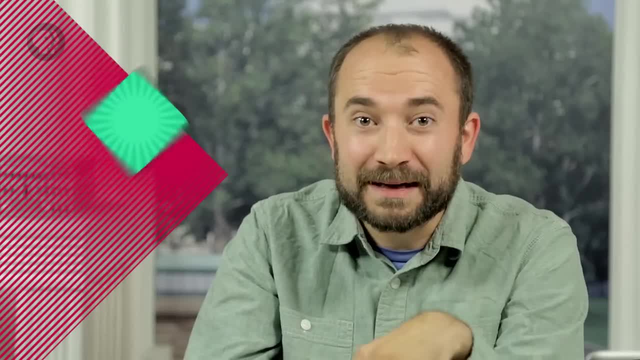 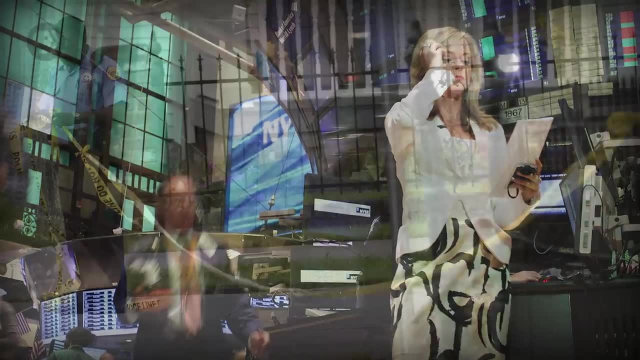 what is called priming. That's when you put a coat of primer on the house before you paint it and the paint sticks real good. No, This is when the media prepares the public to take a particular view of an issue, often through the amount of coverage it gives, For example,